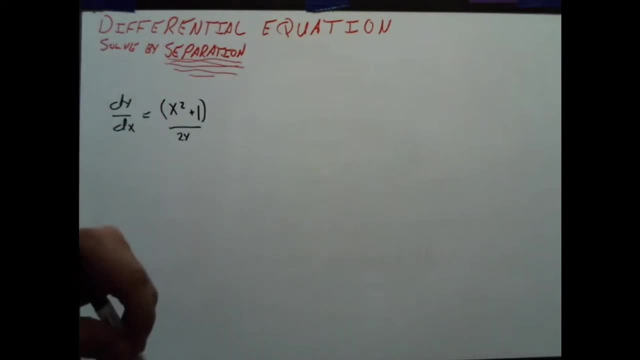 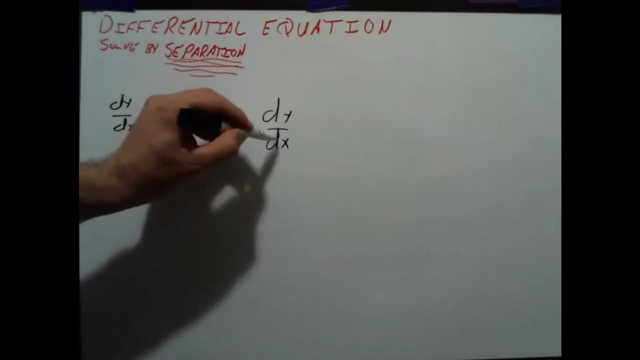 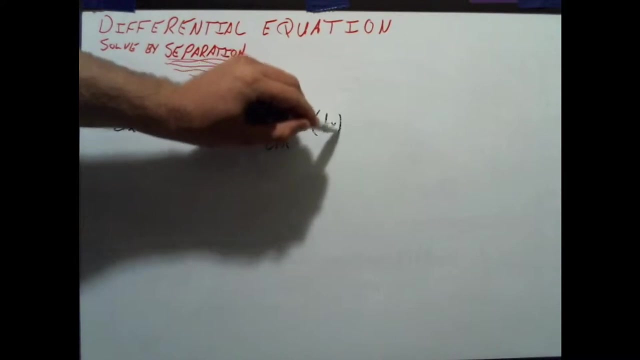 What we're basically saying here is we have the derivative of a function- Let's call it the derivative of the function y, dy, dx- And we use separation of variables when two different functions are being multiplied together. So I'll call it h times g. 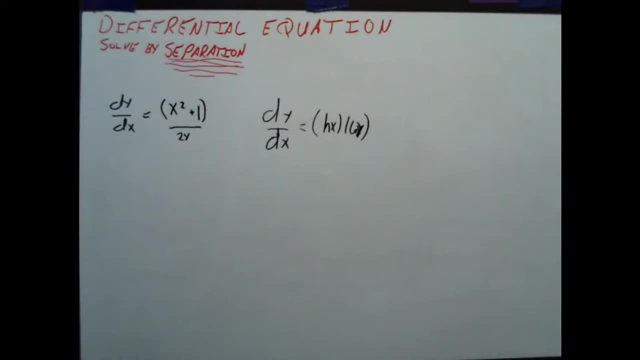 That's better g And it's not too hard of a concept. In fact it's just kind of an exercise in our basic algebra skills. You want to get the x's on one side and the y's on the other. Let me get that g written a little bit neater. 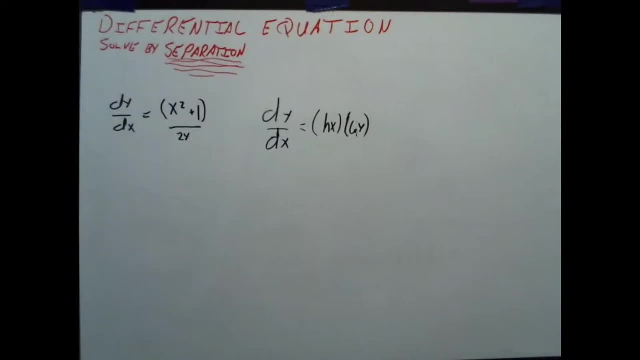 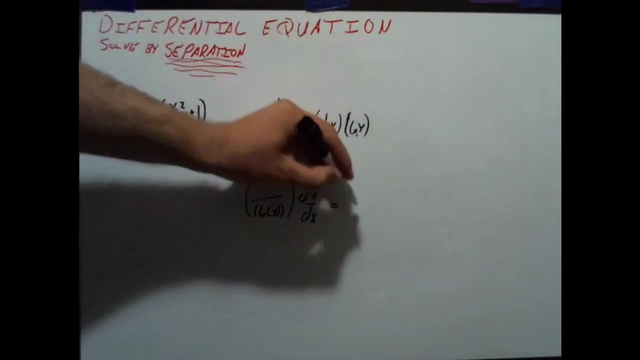 It's kind of hard being left-handed and coming in on the side of the board like this, But I've got h and g, So what I'll do is I'm going to move this g to the other side of the equation And I'll get 1 over g. times dy over dx is equal to h. 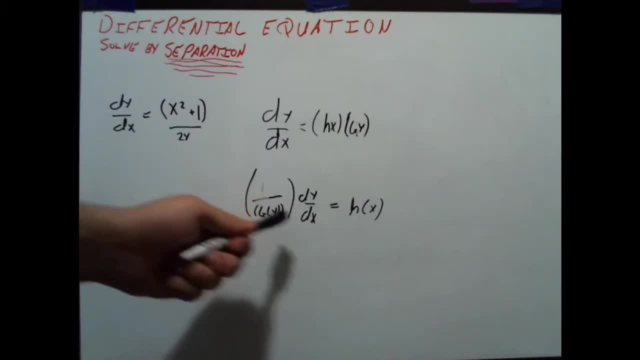 Now I've got y x, y x. So if I multiply my dx to the other side, I'll get 1 over dy over dx, 1 over g dy equals h dx, And that's pretty simple. Well, I started off with the derivative of: a function equals two functions being multiplied together. 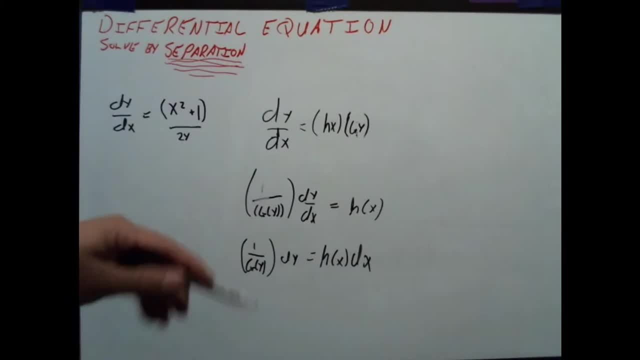 I've separated my variables And now I have to get rid of those annoying dy's and dx's. So I'm going to go ahead and integrate both sides And, doing the integration, integral, integral. we'll get rid of this dx and this dy. 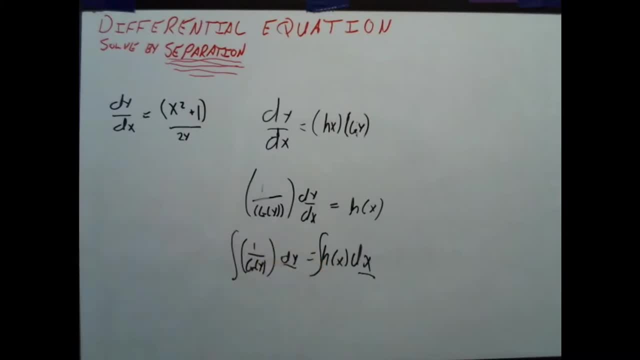 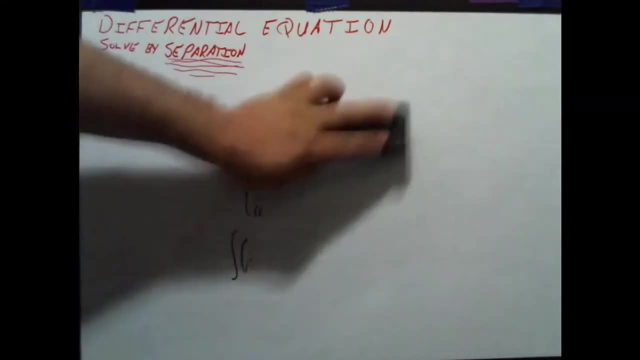 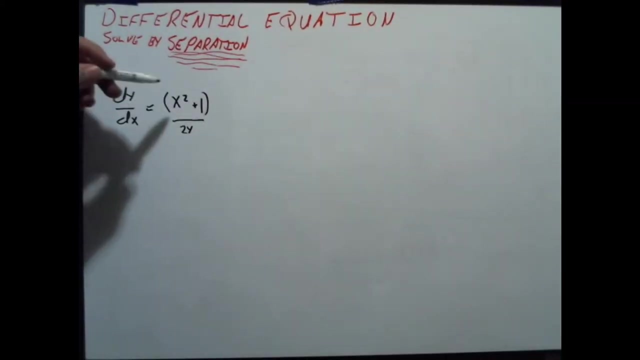 giving me 1 over gy and h integrated, And we can solve for those variables and find that equation. That's the basic, fundamental of what we're going to do. Let's move on to this example. So here we're given: dy over dx equals x squared plus 1 over 2y. 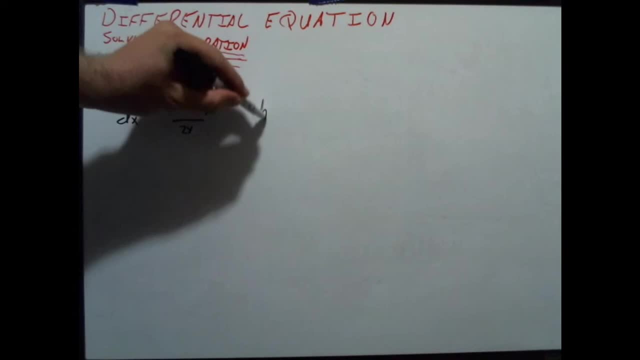 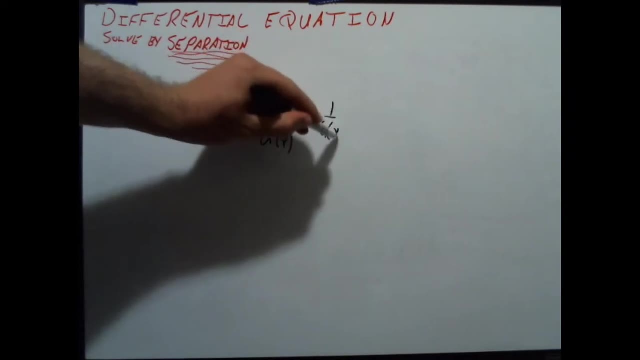 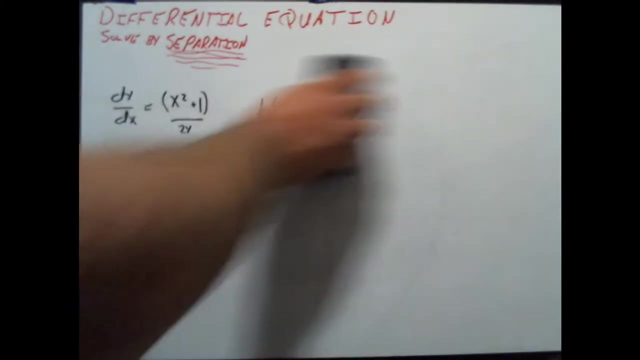 This qualifies because if I have h of x over g of x, that simplifies to 1 over g of x times h of x, So they are being multiplied together in a roundabout way. Division is just the inverse of multiplication. So let's look at this here. 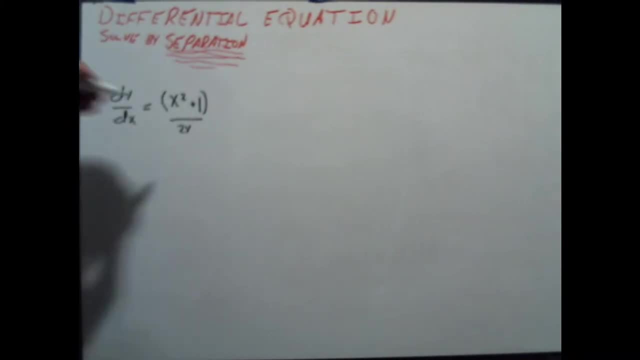 If I move my y's to one side and my x's to one side. that looks easy enough. I'll just multiply by 2y. It's going to be 2y. dy over dx equals x squared plus 1.. Then I multiply my dx over. 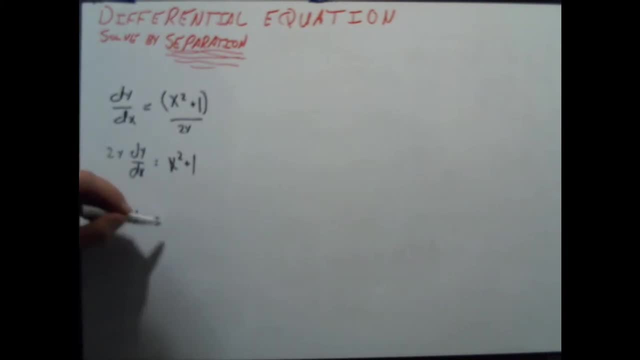 That will give me 2y dy equals x squared plus 1 dx. Now we're all separated. We just have to run some integrals to get rid of those annoying differentials. Aren't they annoying? I think they're terrible, So let's get rid of them. 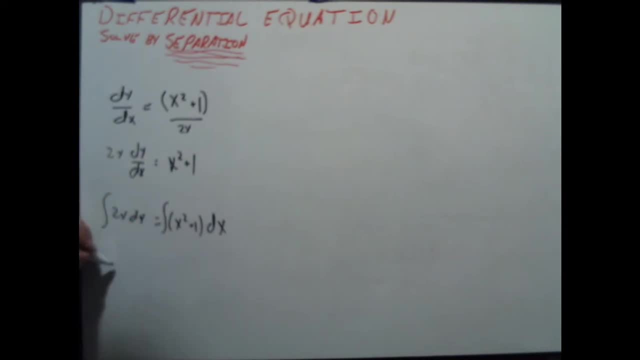 We've got. I've got some integrals there and I'm going to say y squared equals x, cubed over 3 plus x. And then I'm going to add on a plus c, because we've just integrated I do not put a plus c on the y side. 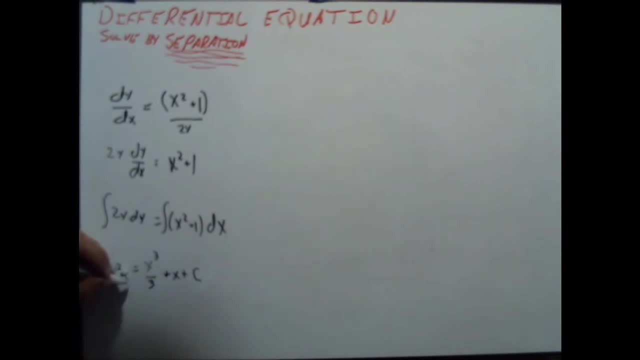 If you're wondering why, it's because I could say plus c. and then let's say I put a little y script there, x subscript here. Well, on my next step, I would say minus c of y to cancel them out and get the c's on both sides. 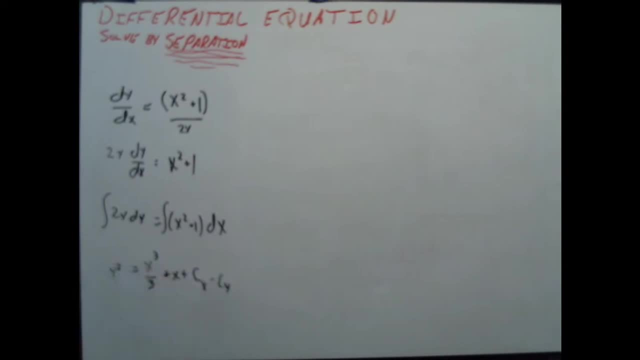 And this is just some arbitrary number, because our c's are arbitrary numbers, So it's only necessary to put a c on one side. Now, if I- This is a perfectly acceptable differential equation solution- I could want to have a y equals. 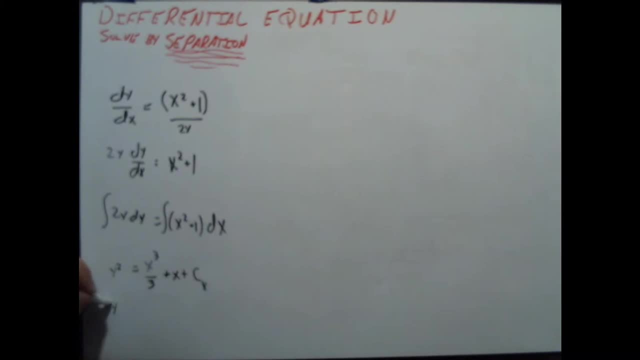 if that be the case, it's not too bad. I say y equals and then I square root both sides plus or minus. that was bad. plus or minus signs. plus or minus square root of x cubed over 3 plus x plus c.